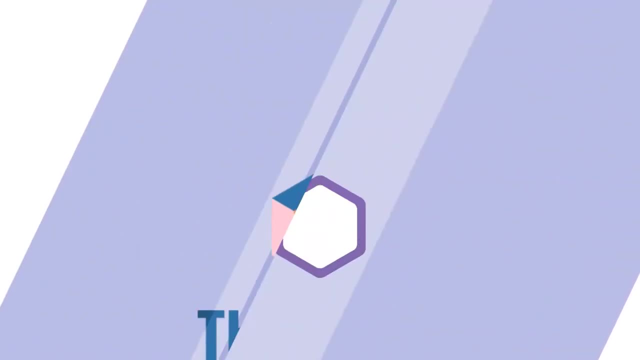 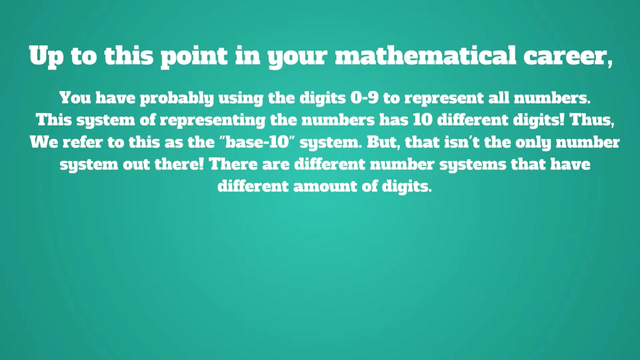 This video is brought to you by ThePuzzlercom. Up to this point in your mathematical career, you have probably used the digits 0 to 9 to represent all numbers. This system of representing the numbers has 10 different digits. Thus, 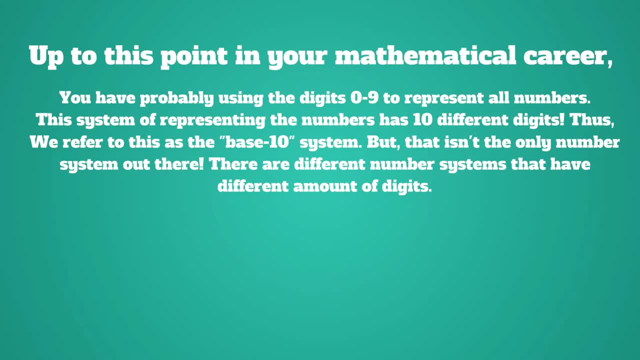 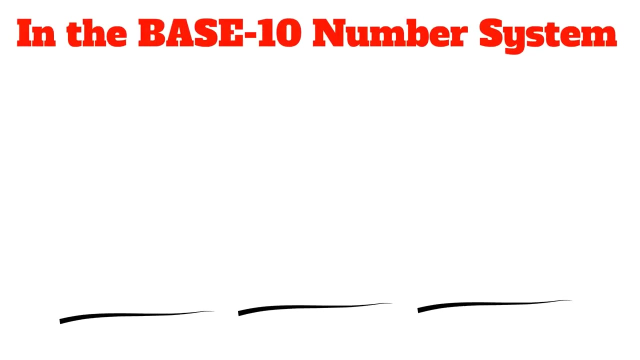 we refer to this as the base 10 system, But that isn't the only number system out there. There are different number systems that have different amount of digits. For example, in the base 10 number system, the number 234 is equal to starting all the. 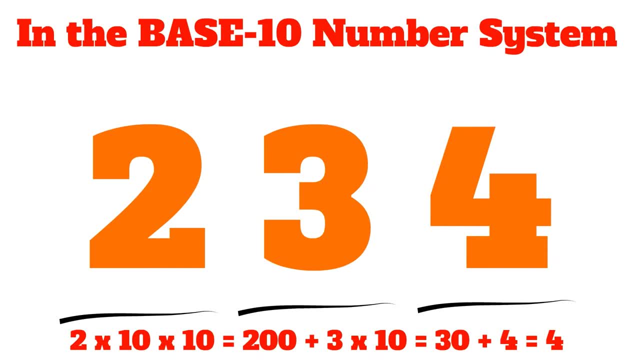 way from the left, 2 times 10 times 10,, because that's the third digit from the right. Then the second digit is the 3, and since that's the second digit, we multiply it by 10 to the power of 1.. 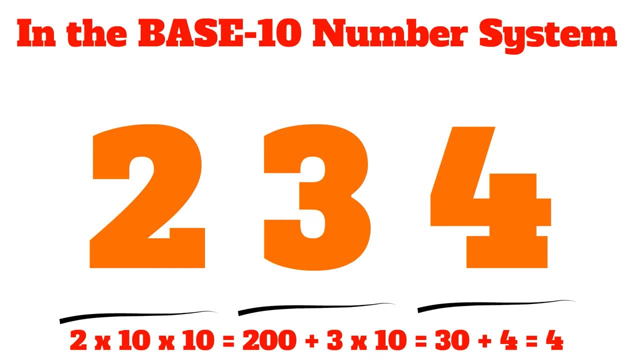 That gives us 30.. Finally, the third digit, or the first digit from the right, is multiplied by 10 to the power of 0, which is 1, so 4 times 1 gives us 4.. Thus the number 234 is. 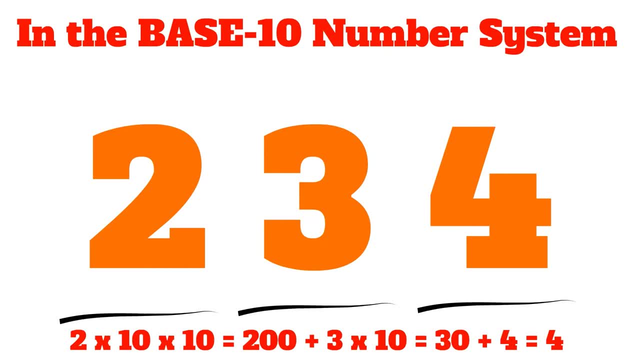 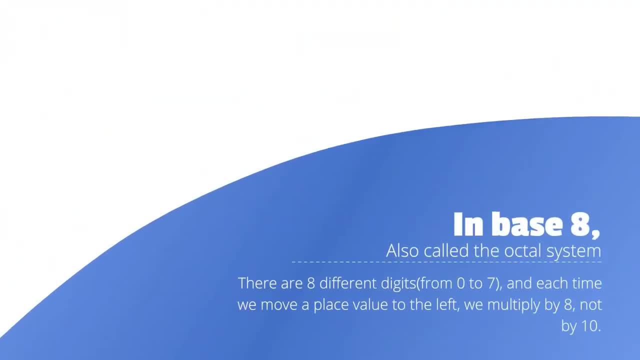 just equal to 200 plus 30 plus 4, or 234 in base 10.. It'll make more sense when we look at other bases. Here's another example. In base 8, also called the octal system, there are 8 different digits. 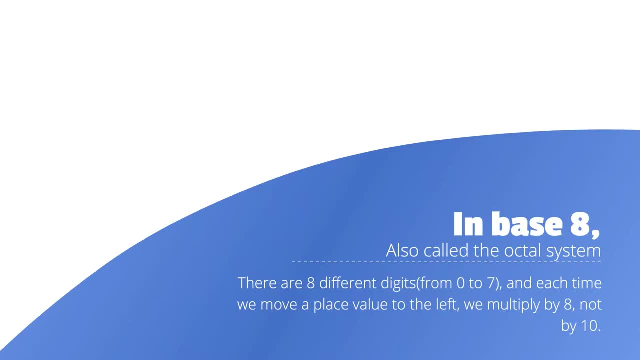 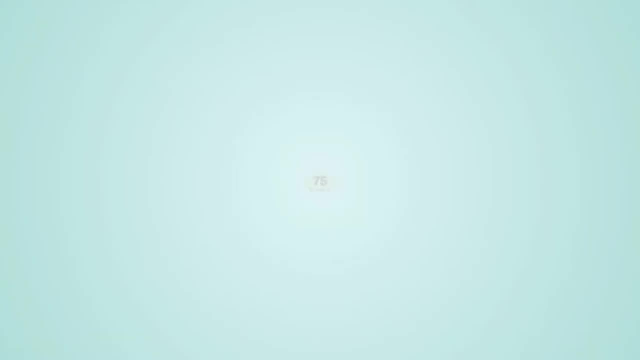 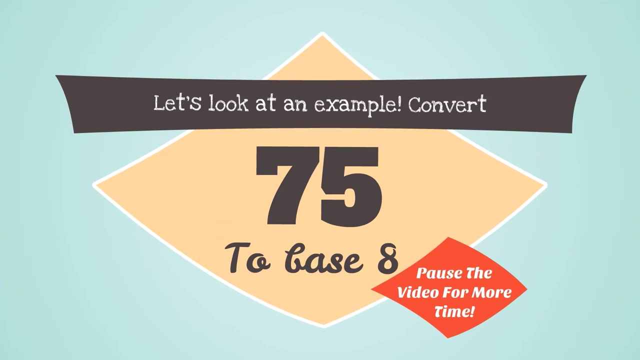 from 0 to 7.. And each time we move a place value to the left, we multiply by 8, not by 10.. Let's look at an example: Convert 75 to base 8.. Pause the video if you want more time on. 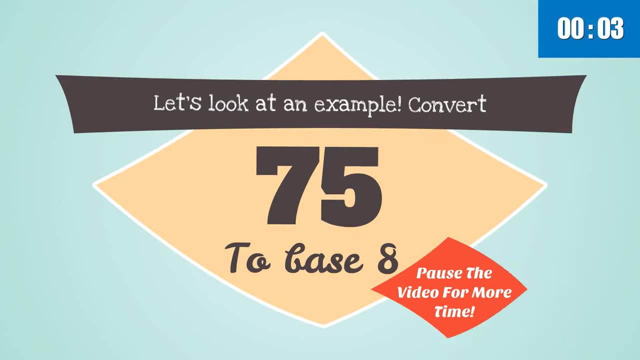 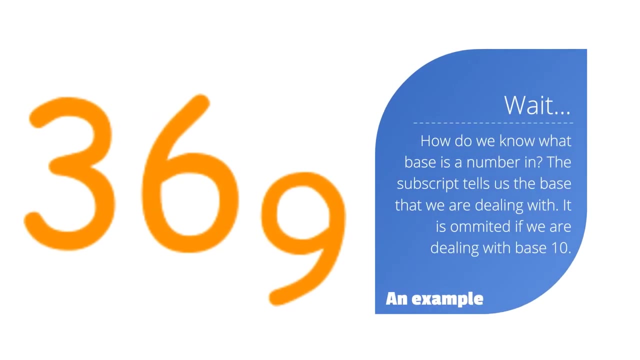 this question. Wait, How do we know what base a number is in The subscript tells us the base that we are dealing with, And we omit this if we are dealing with base 10.. For example, here we have 36 with a subscript of 9, which means that we 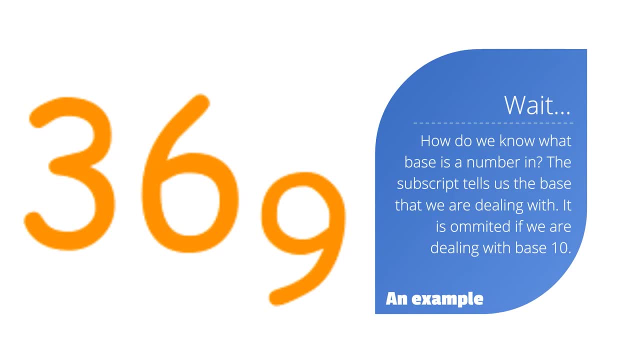 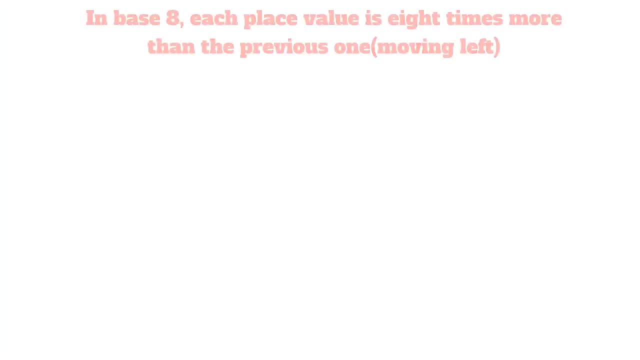 are dealing with 36 in base 9.. If, instead, I just had the number 36 here, we would know that we are dealing with 36 in base 10.. Let's look at another example. In base 8, also called the octal system, there are 8. 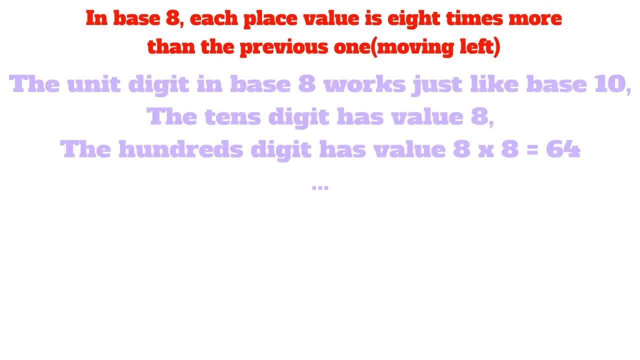 places In base 8,. each place value is 8 times more than the previous one as we move to the left. So the unit digit in base 8 works just like base 10.. The tenths digit has a value of 8,. 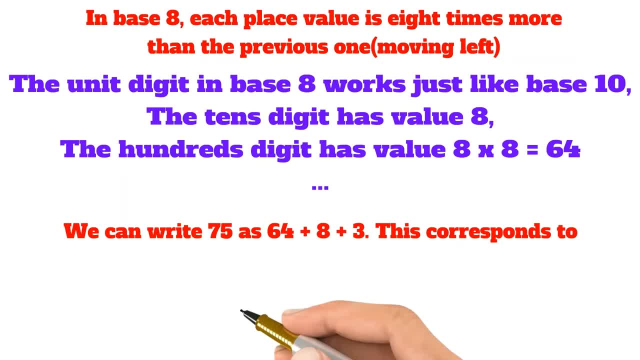 so whatever is in the tenths digit is multiplied by 8.. The hundredths digit has a value of 8 times 8, or 8 squared or 64. So whatever is in the hundredths digit, we multiply that by 64. And so on. 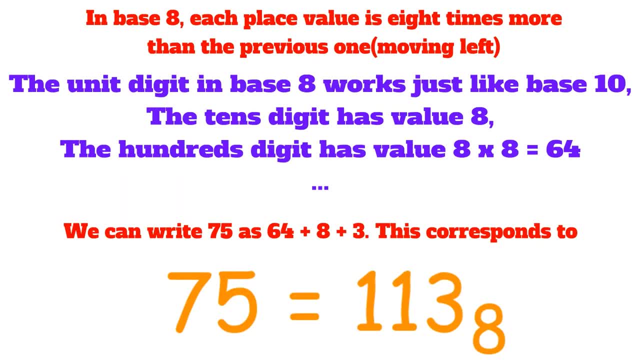 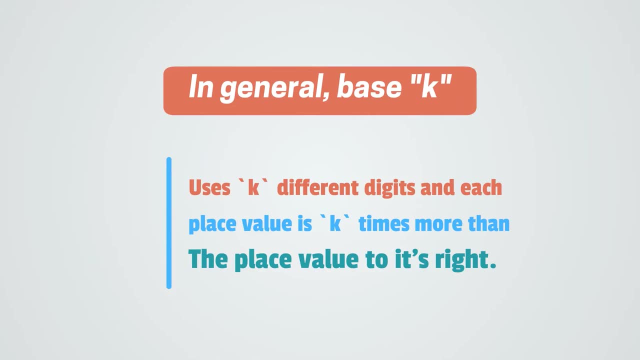 We can then write 75 as 64 plus 8 plus 3.. Now this is 1, 100 in octal base, 1 tens and 3 ones. so 75 is equal to 113 in base 8.. In general, base k uses k different digits and each place value is k times more than. 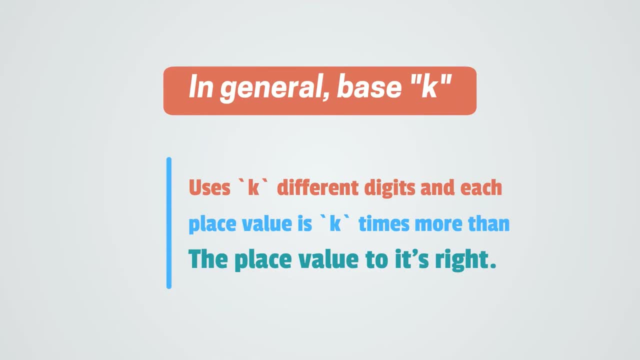 the place value to its right. The place value all the way to the right is k to the power of 0, or 1, and the place value to the left would be k. the place value to the left of that would be k squared, and so on. 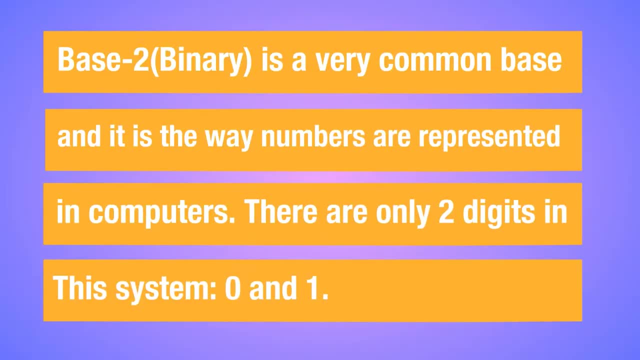 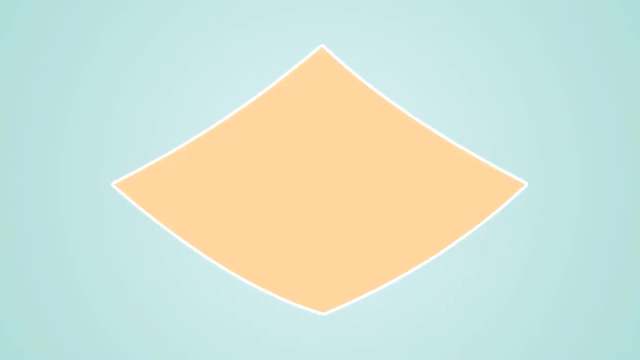 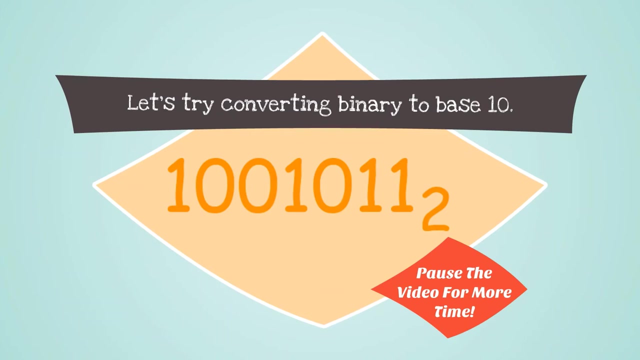 Base 2, also known as binary, is a very common base and it is the way numbers are represented in computers. There are only 2 digits in this system: 0 and 1.. Let's try converting binary to base 10.. Convert 1 million, 1 thousand and 11 in base 2 to 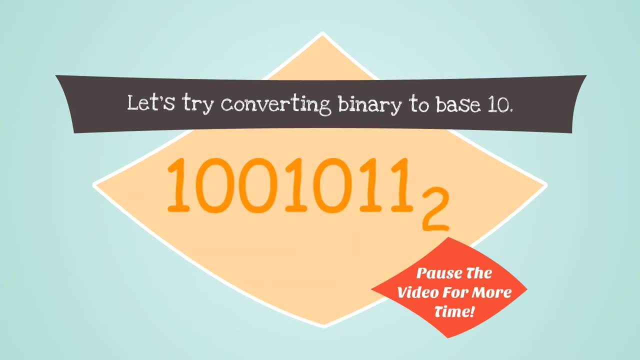 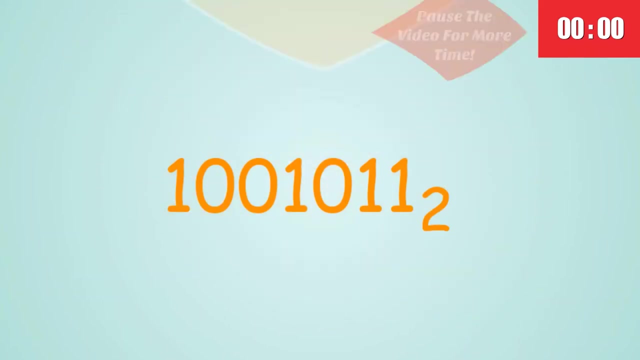 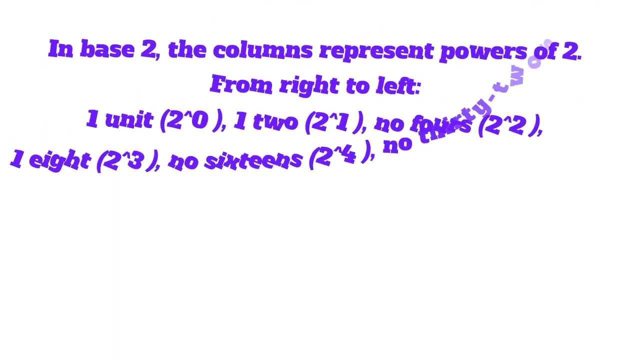 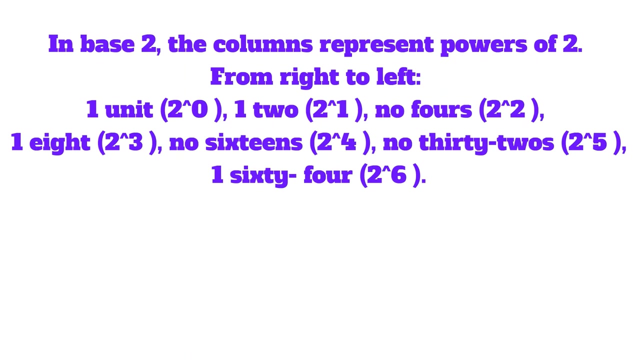 base 10.. Pause the video if you'd like more time on this question. In base 2, the place values represent powers of 2.. Starting from the right to left, we have 1 unit or 2 to the power of 0,. 1, 2,, no, 4s. 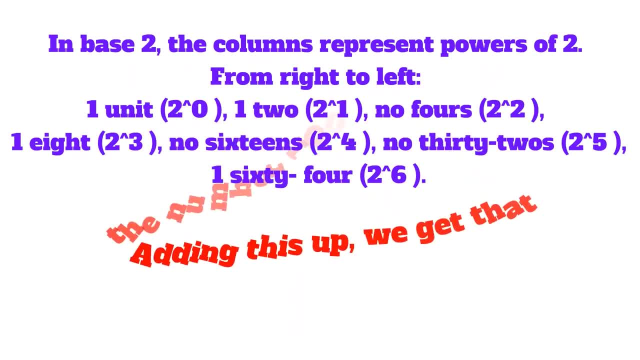 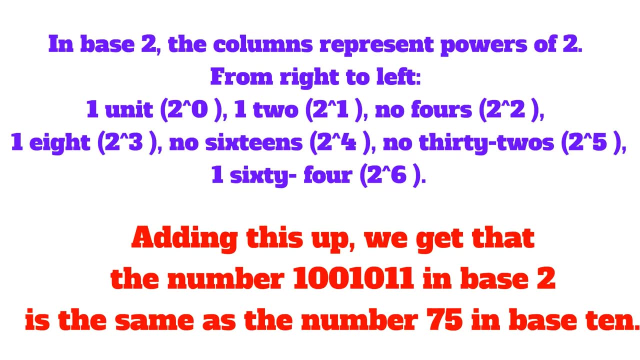 1 8s, no 16s, no 32s and 1 64. Adding this up, we get that the number 1001011 in base 2 is the same as the number 75 in base 10.. 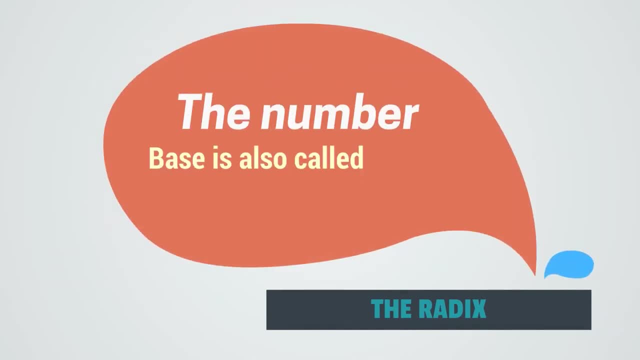 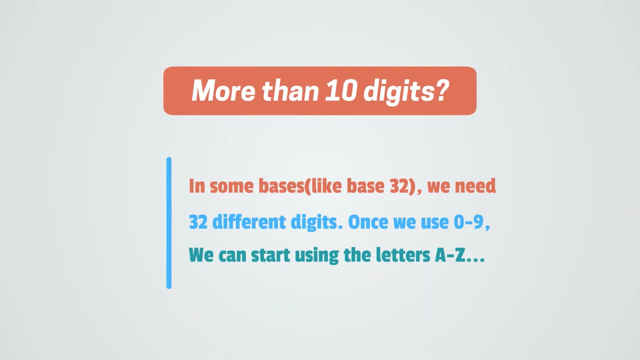 The number base is also called the radix. An interesting question now arises: what if we have more than 10 digits? In some bases, like base 32,, we have more than 10 digits. In some bases, like base 32,, we have more than 10 digits. 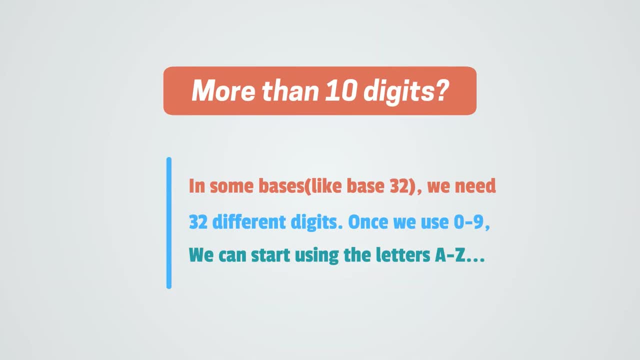 So we actually need 32 different digits. Well, once we use the digits 0 to 9, we move on to the letters A through Z, And if we ever finish with those, we have more symbols that we can use after that, although 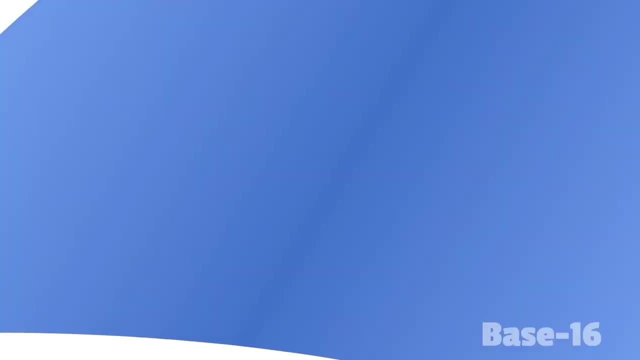 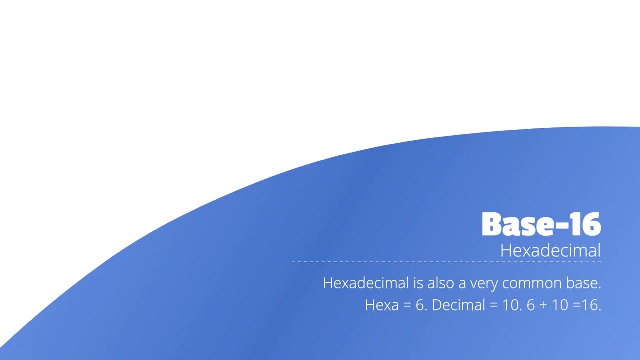 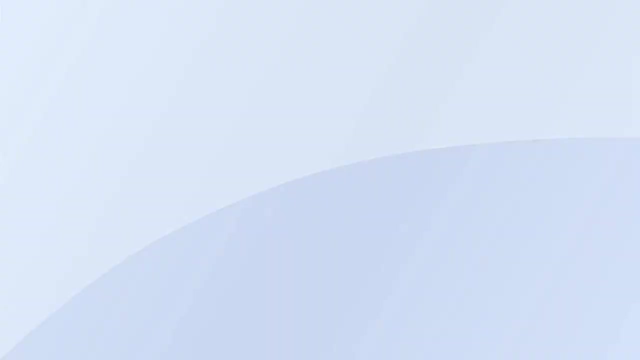 they are usually not needed. Base 16, also known as a hexadecimal base, is also a very common base. Hexa means 6 and decimal means 10.. Adding up 6 plus 10 gives us base 16.. Converting bases: We frequently have to convert bases. What is the easiest way to do that? 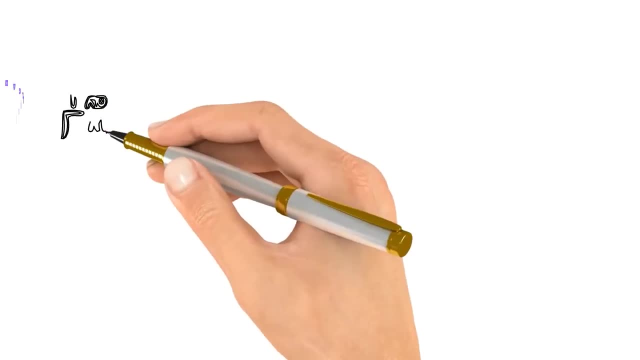 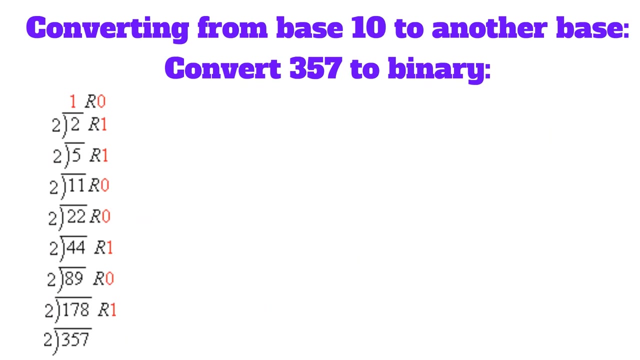 Let's take a look Converting from base 10 to another base. Let's convert 357 to binary. Now here is the process we follow: We divide the number that we have- 357, to the base that we want to make it, or. 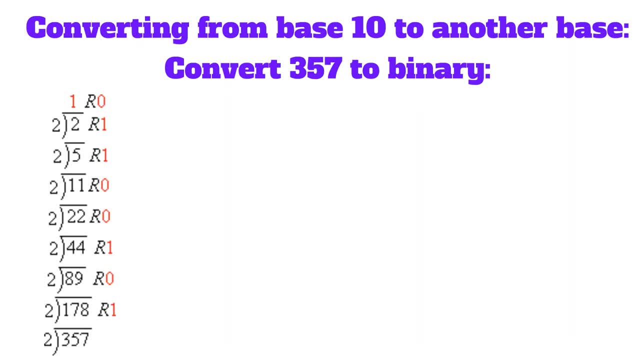 convert it to, For example. in this case we want to convert to base 2.. So we do 357 divided by 2. That gives us 178 with a remainder of 1.. Once again, we divide 178 by 2. That. 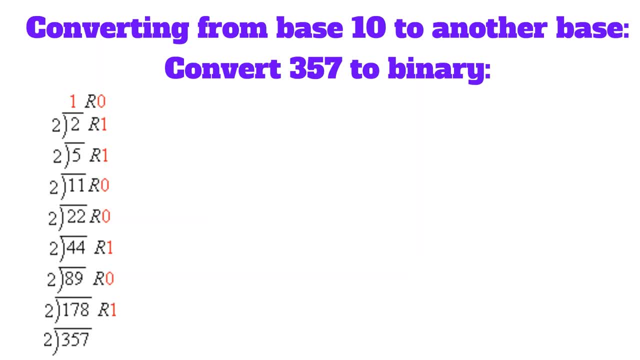 gives us 89 with a remainder of 0. We divide that by 2 again to get 44 with a remainder of 1.. And going on, we get 22 with a remainder of 0,, 11 with a remainder of 0,, 5 with a remainder. 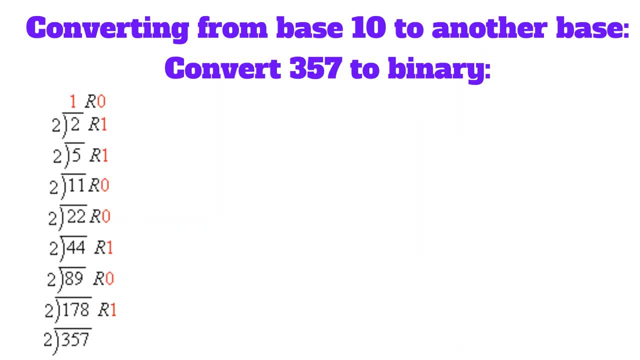 of 1, and then 2 with a remainder of 1, and finally 1 with a remainder of 0.. Converting from base 20 to another base. Let's see how we convert this to binary. Let's Now: this number just converts to 1 0, 1, 1 0, 0, 1 0, 1 in base 2.. 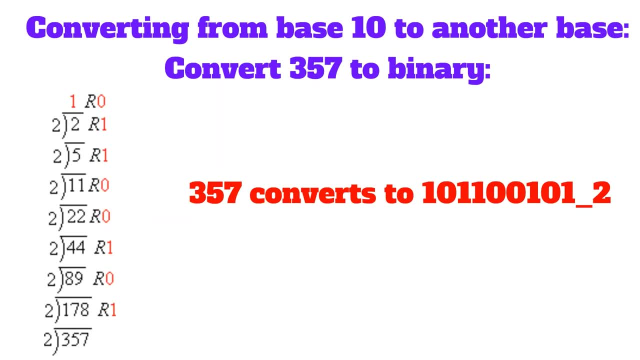 The way we found that out was we read the topmost quotient and then we just read all the remainders going down. In fact, this method works in any base. So 357 converts to 1 0, 1, 1 0 0, 1 0 1 in base 2.. 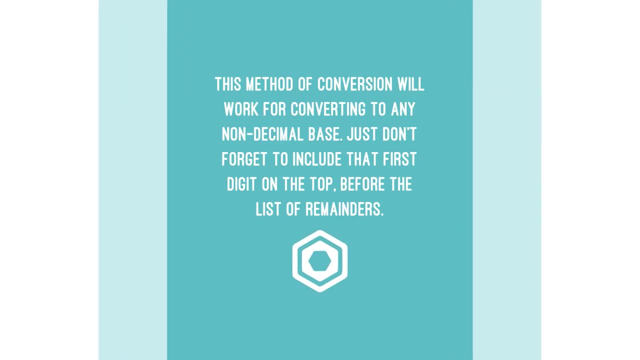 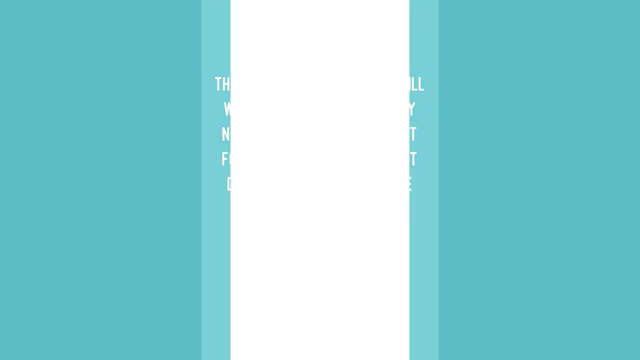 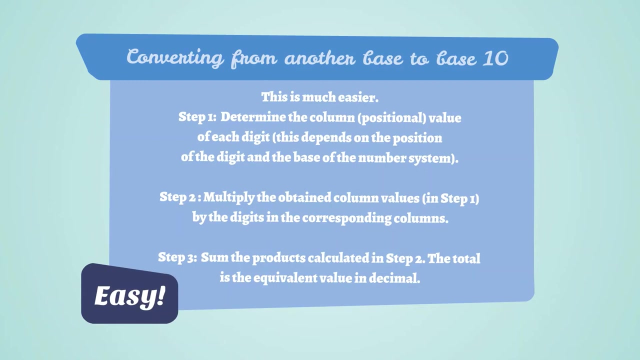 This method of conversion will work for converting to any non-decimal base. Just don't forget to include that first digit on the top before the list of remainders Converting from another base to base 10, or the decimal base. This is much easier. 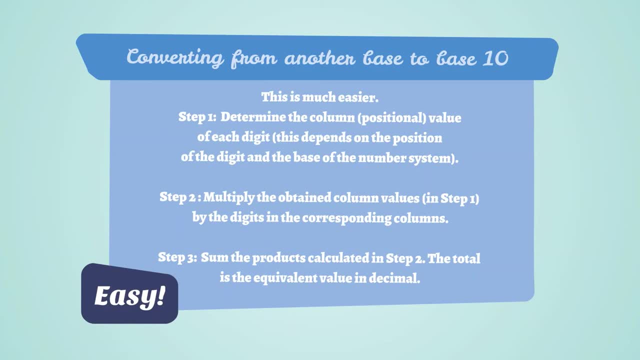 There are 3 steps to this. Step 1. Determine the column or place value or the positional value of each digit. This depends on the position of the digit and the base of the number system. Step 2. Multiply the obtained column values in step 1 by the digits in the corresponding columns. 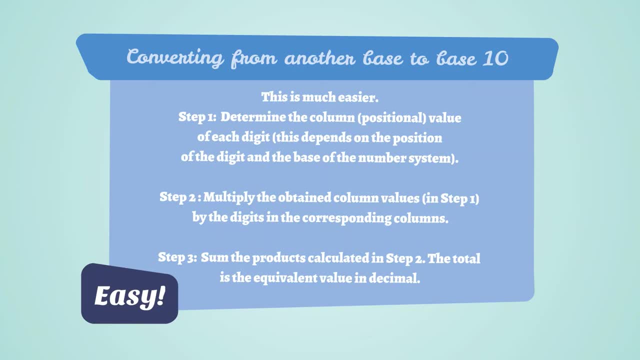 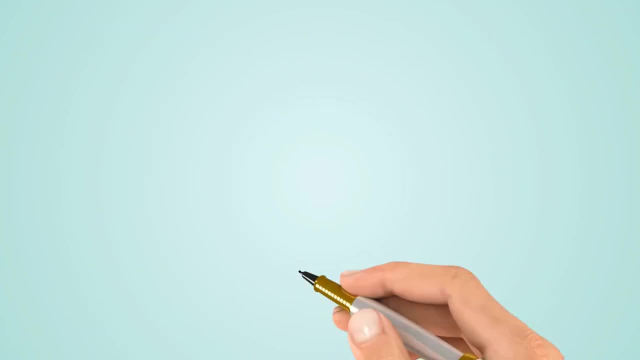 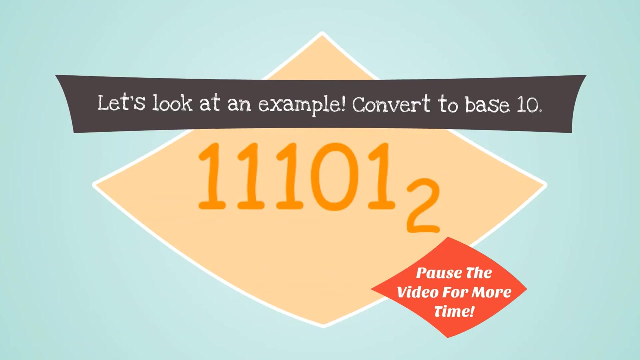 Step 3.. Sum the products calculated in step 2.. The total is the equivalent value in decimal. Let's take a look at an example for this method. Let's look at an example: Convert to base 10.. 11,101 in base 2.. 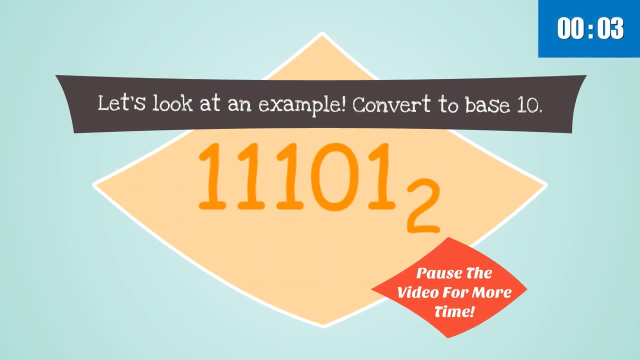 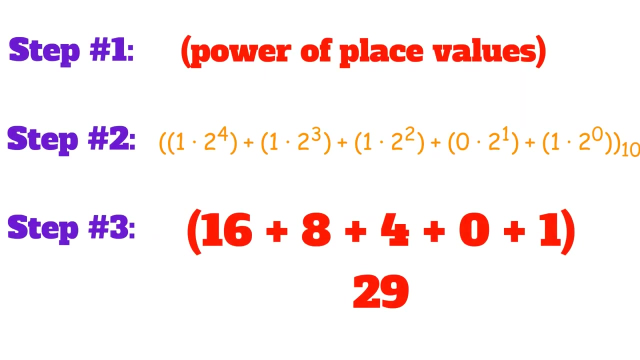 Pause the video. if you want more time on this question, Let's follow our 3 steps. Step number 1 is determining the power of the place values. Well, starting all the way to the right, It's the units place value. Then, moving to the left, we have 2 to the power, 1, or 2.. 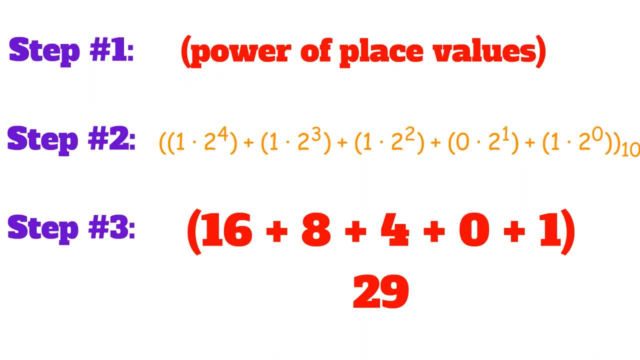 Moving again to the left is 2 squared or 4.. Moving to the left again is 2 cubed or 8.. Moving to the left again and for the last time, is 2 to the power, 4, or 16.. 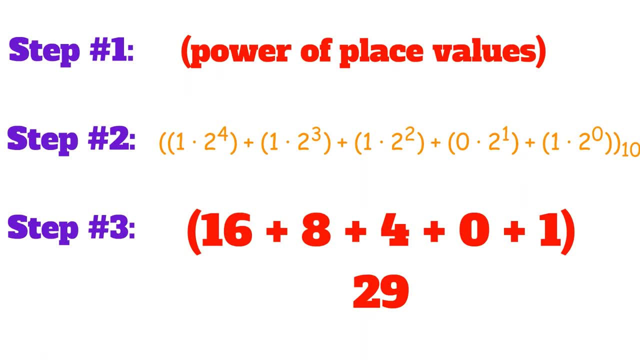 Now step number 2 is multiplying each of the digits in each place value by the power of that place value. Starting all the way from the left, we have 1 times 2 to the power, 4 plus 1 times 2 to the power, 3 plus 1 times 2 squared, plus 0 times 2 to the power, 1 plus 1 times 2 to the. 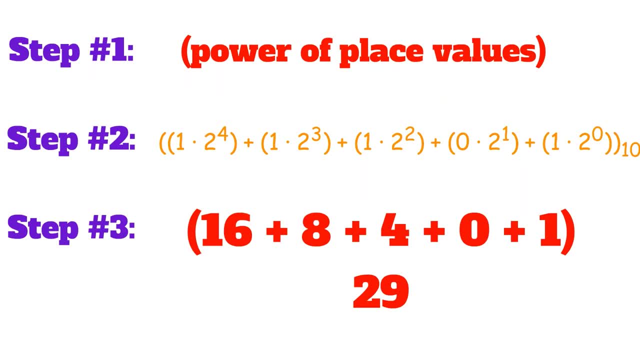 power 0.. And remember, this product or this sum is in base 10.. Now, converting each of the single terms to base 10, we get 16 plus 8 plus 4 plus 0 plus 1, which gives us 29 in base 10..